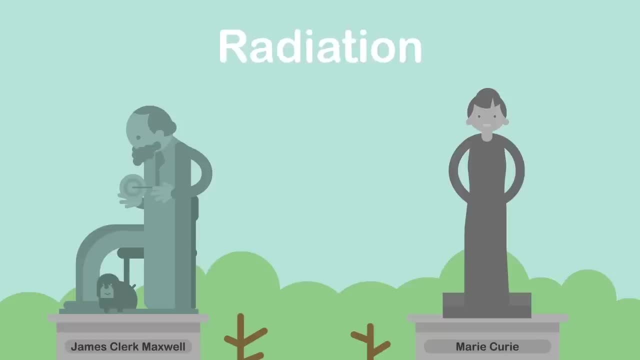 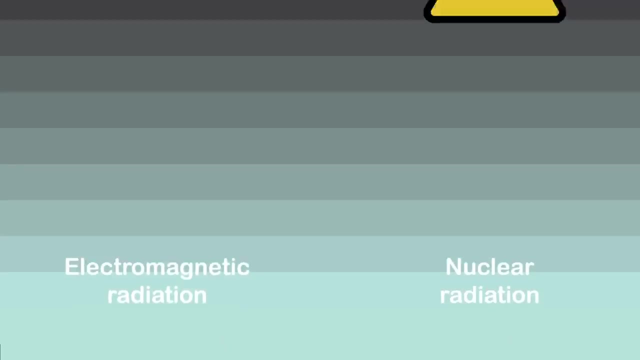 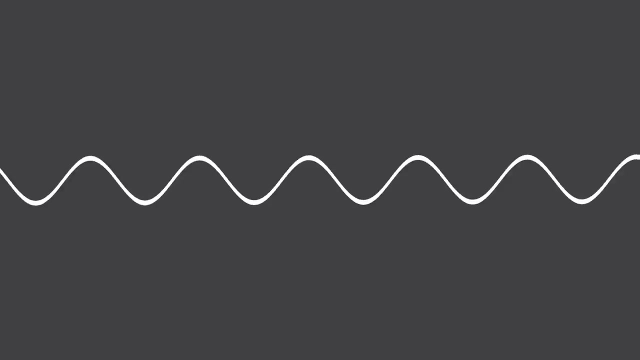 The answer begins with understanding that the word radiation describes two very different scientific phenomena: electromagnetic radiation and nuclear radiation. Electromagnetic radiation is pure energy consisting of interacting electrical and magnetic waves oscillating through space. As these waves oscillate faster they scale up in energy. 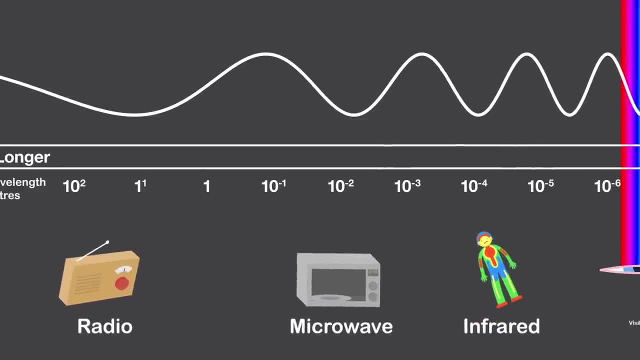 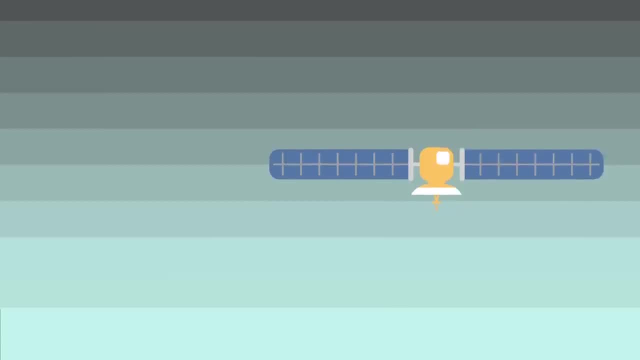 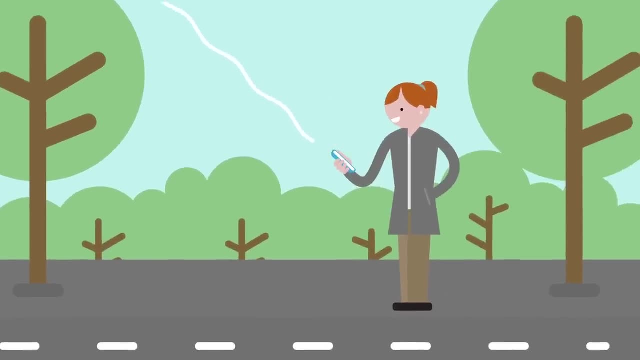 At the lower end of the spectrum there's radio, infrared and visible light. At the higher end there are ultraviolet, x-ray and gamma rays. Modern society is shaped by sending and detecting electromagnetic radiation. We might download an email to our phone via radio waves. 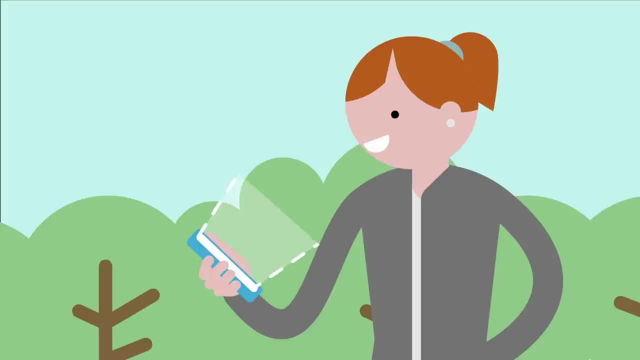 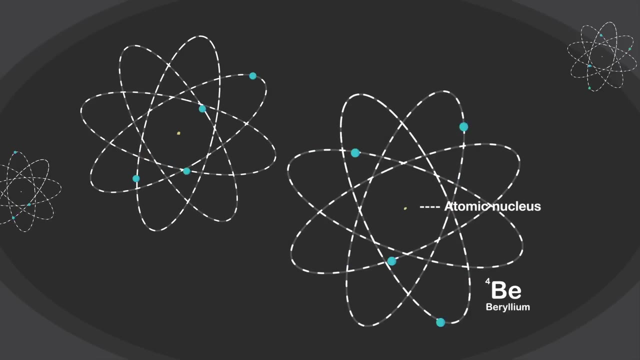 to open an image of an x-ray print, which we can see because our screen emits visible light. Nuclear radiation, on the other hand, originates in the atomic nucleus, where protons repel each other due to their mutually positive charges, A phenomenon known as. 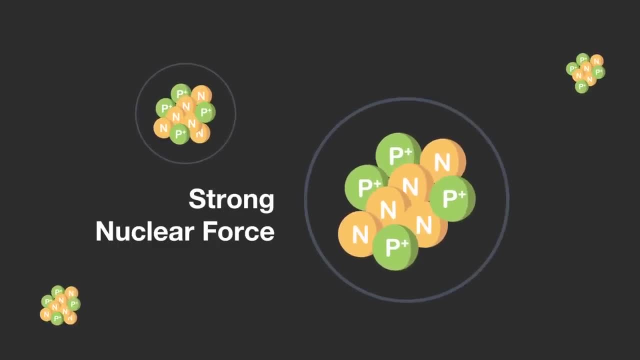 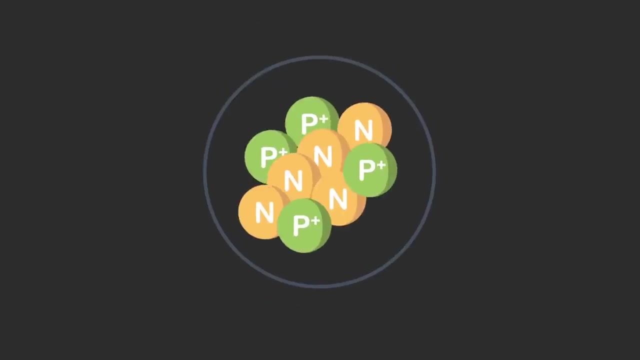 the strong nuclear force struggles to overcome this repulsion and keep the nucleus intact. However, some combinations of protons and neutrons, known as isotopes, remain unstable or radioactive. They will randomly eject matter and or energy, known as nuclear radiation, to achieve greater stability. 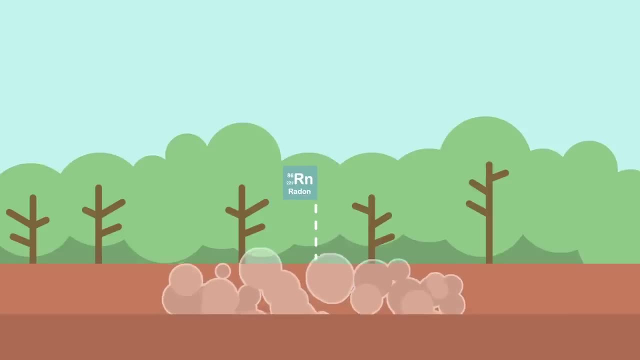 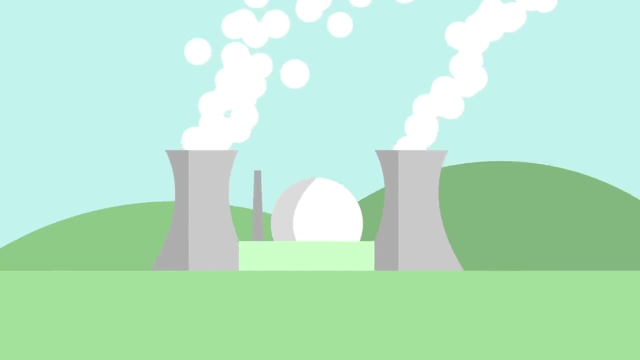 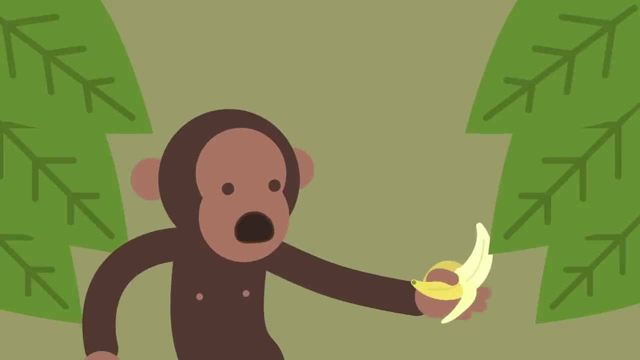 Nuclear radiation comes from natural sources like radon, a gas which seeps up from the ground. We also refine naturally occurring radioactive ores to fuel nuclear power plants. Even bananas contain trace amounts of a radioactive potassium isotope. So if we live in a world of radiation, 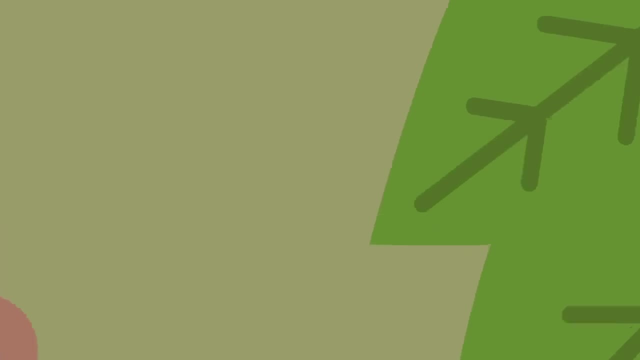 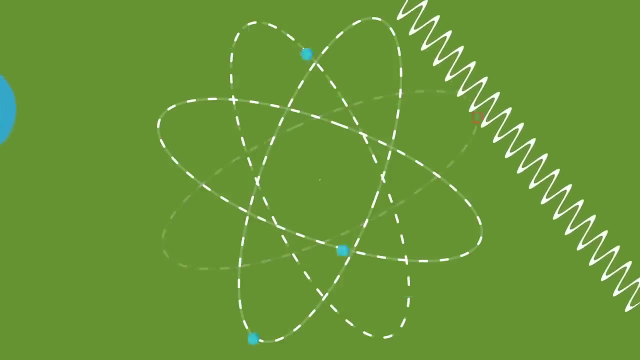 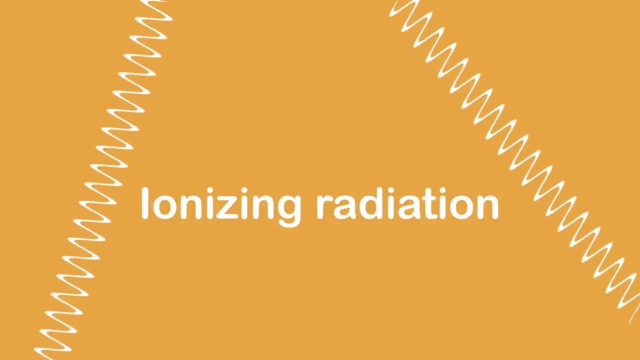 how can we escape its dangerous effects? To start, not all radiation is hazardous. Radiation becomes risky when it rips atoms' electrons away upon impact, a process that can damage DNA. This is known as ionizing radiation, because an atom that has lost or gained electrons is called an ion. 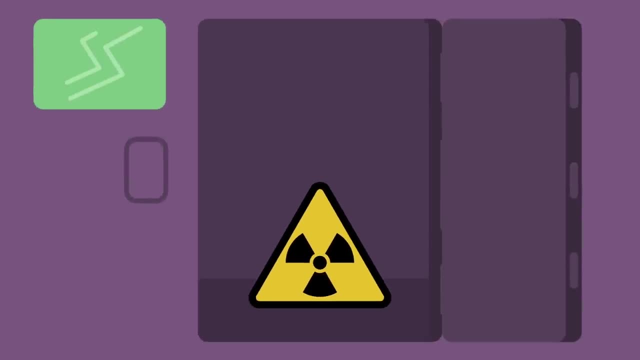 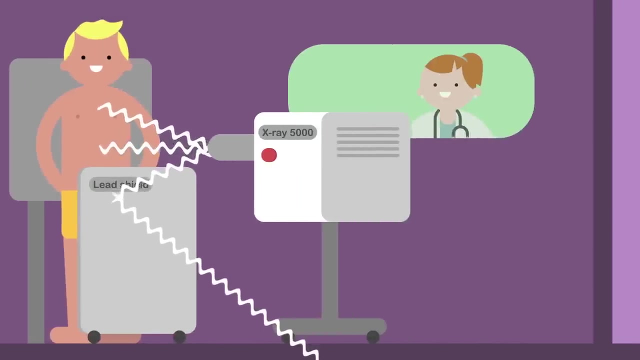 All nuclear radiation is ionizing, while only the highest energy electromagnetic radiation is. That includes gamma rays, X-rays and the high-energy end of ultraviolet. That's why, as an extra precaution, during X-rays, doctors shield body parts they don't need to examine.